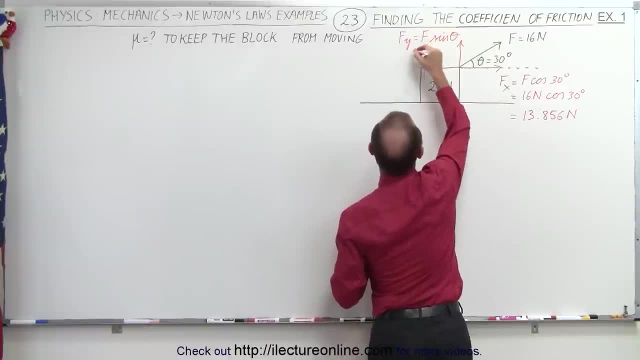 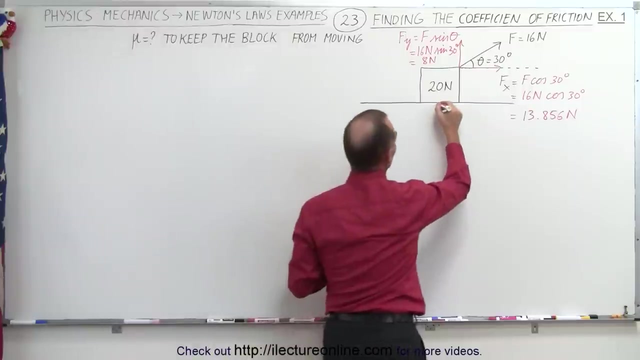 f times the sine of theta, and so it would be 16 newtons. So that's equal to 16 newtons times the sine of 30 degrees, which is equal to 0.5 or 8 newtons. We also have to think about the force of the weight acting on the block, So we have a force pulling. 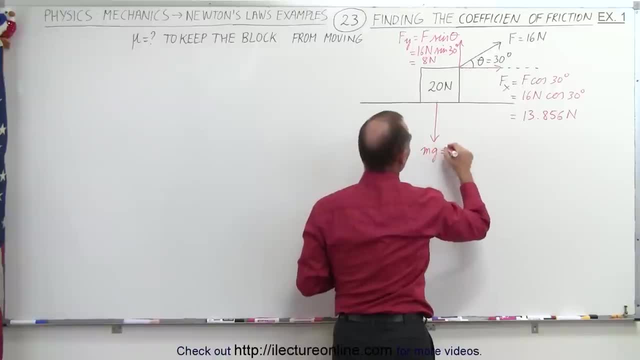 down. So it would be mg, and in this case that's equal to 20 newtons. And then there's a normal force pushing back. Now here we have to be careful about the normal force. The normal force is not going to be equal to mg in this case, because there's also a force here that's partially pulling. 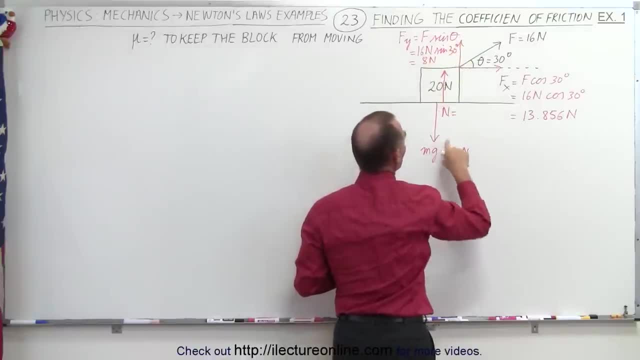 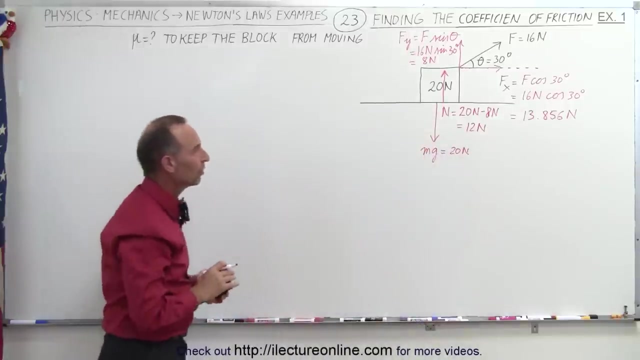 up on the block with a force of 8 newtons. So therefore the normal force will be 20 newtons minus the 8 newtons from this force. So 20 newtons minus 8 newtons, which is therefore 12 newtons. So the normal force is only 12 newtons in this case. Now we also have a friction force. 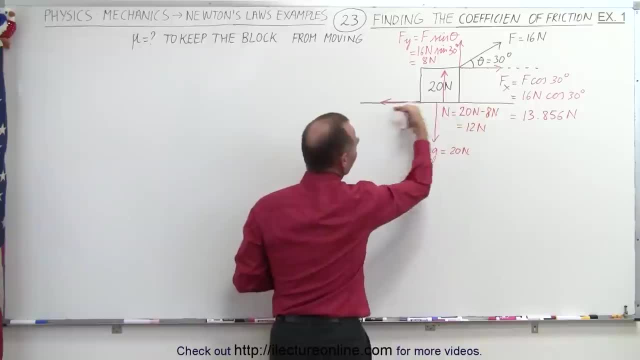 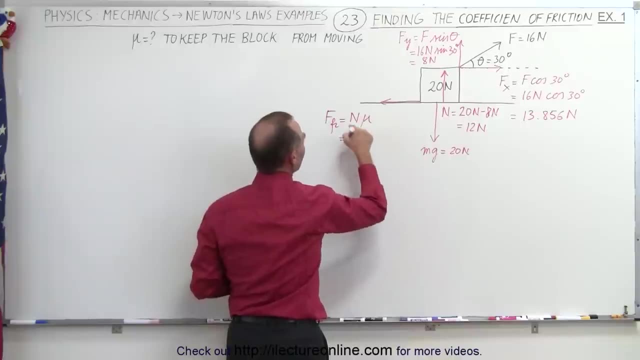 acting on this, Since the block is being pulled in that direction, the friction force will be an opposing force, So the friction force in this case is equal to the normal force times mu. In this case, the normal force will be 12 newtons times mu, And of course we're trying to 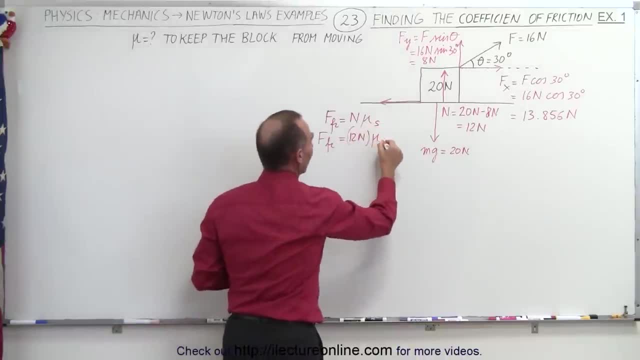 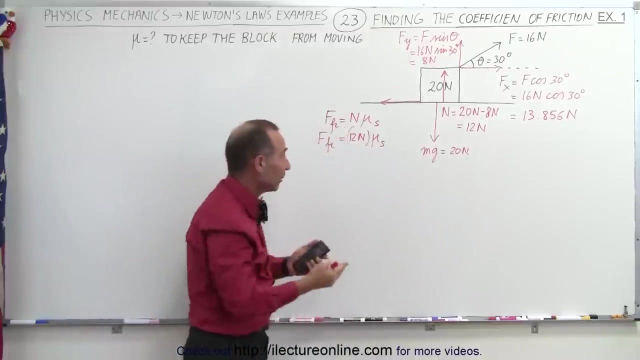 find the value for mu. And, yes, let's call it the static coefficient of friction. So if the friction force is going to prevent the block from sliding to the right from the block to begin to move, the friction force, the maximum friction force you can have, because 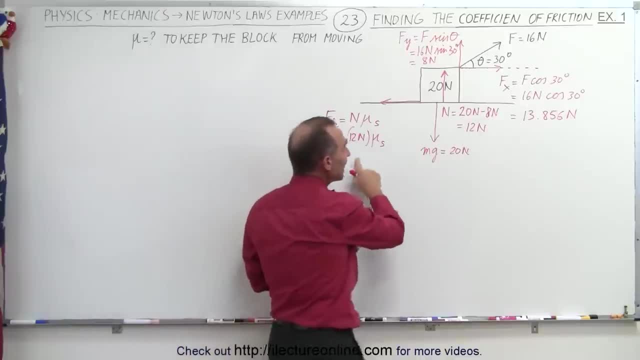 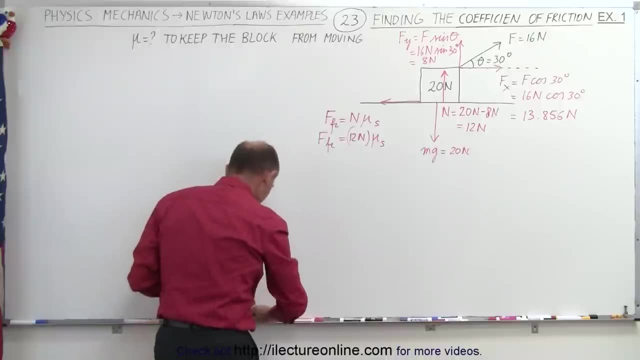 essentially, this is the maximum friction. force must be at least equal to the force in the x direction which we have right here. So what we're looking for is- and let me grab my black pen now- So what we want is to want the force, friction, to be greater than. 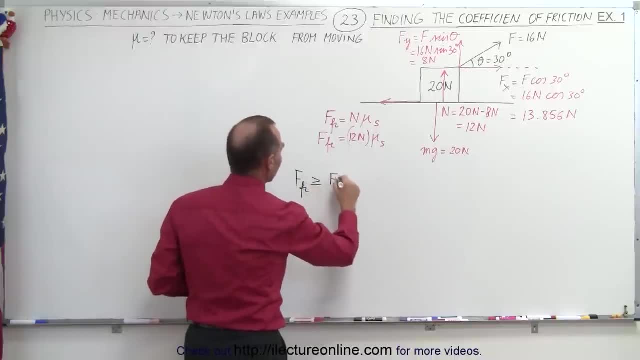 or equal to the force in the x direction that's applied And our friction force. we now know that's equal to 12 newtons times the coefficient of static friction And that must be greater than or equal to f sub x, which is 13.8.. 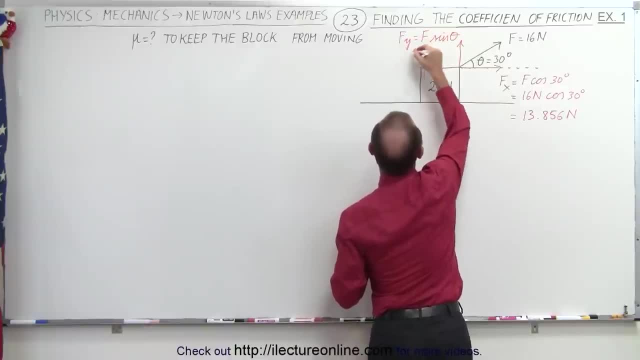 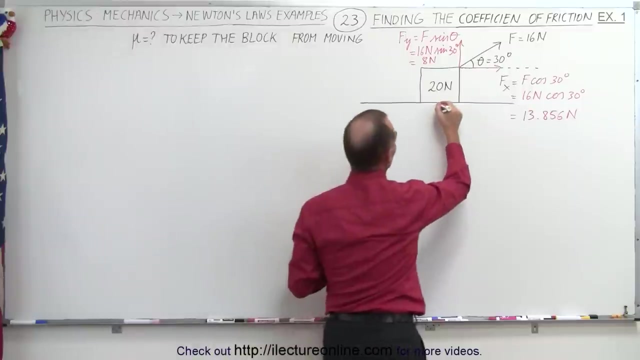 f times the sine of theta, and so it would be 16 newtons. So that's equal to 16 newtons times the sine of 30 degrees, which is equal to 0.5 or 8 newtons. We also have to think about the force of the weight acting on the block, So we have a force pulling. 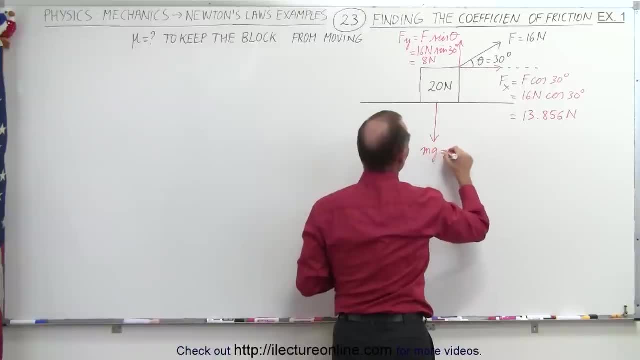 down. So it would be mg, and in this case that's equal to 20 newtons. And then there's a normal force pushing back. Now here we have to be careful about the normal force. The normal force is not going to be equal to mg in this case, because there's also a force here that's partially pulling. 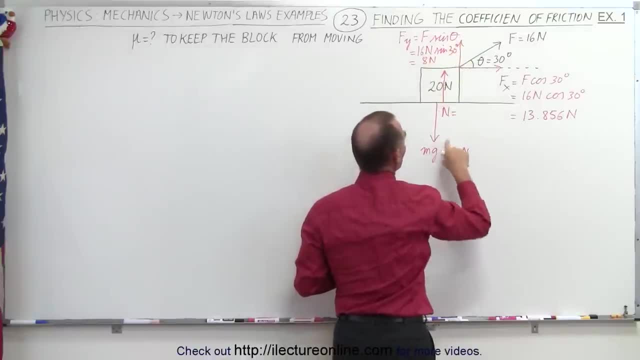 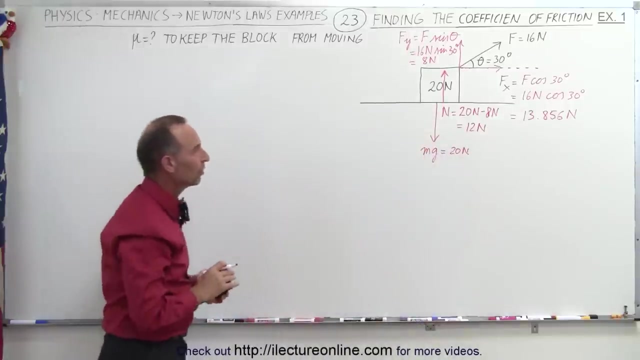 up on the block with a force of 8 newtons. So therefore the normal force will be 20 newtons minus the 8 newtons from this force. So 20 newtons minus 8 newtons, which is therefore 12 newtons. So the normal force is only 12 newtons in this case. Now we also have a friction force. 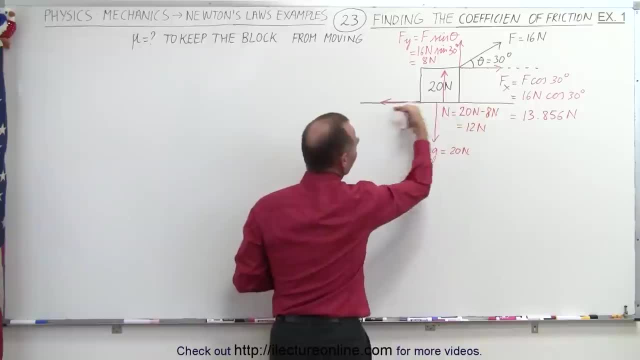 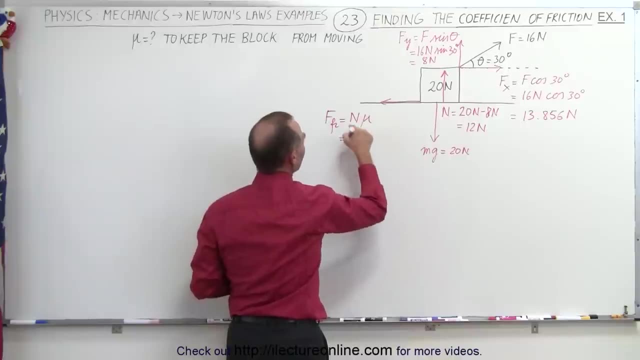 acting on this, Since the block is being pulled in that direction, the friction force will be an opposing force, So the friction force in this case is equal to the normal force times mu. In this case, the normal force will be 12 newtons times mu, And of course we're trying to 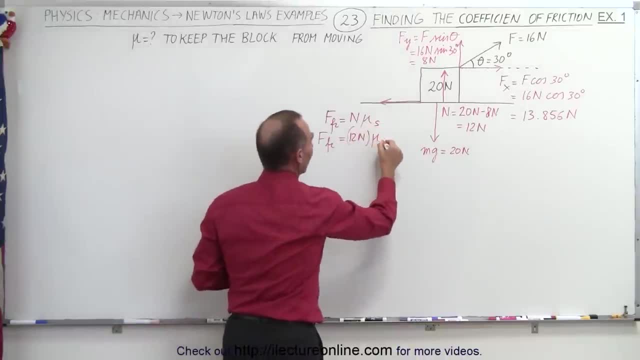 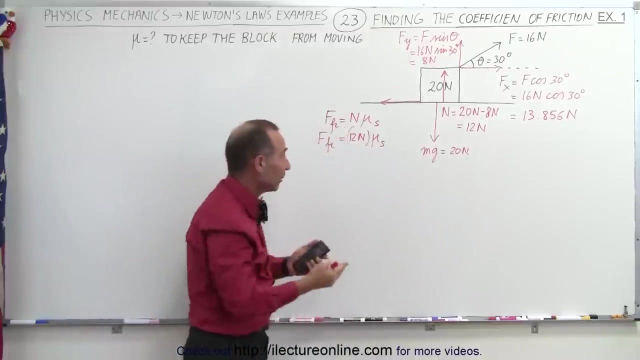 find the value for mu. And, yes, let's call it the static coefficient of friction. So if the friction force is going to prevent the block from sliding to the right from the block to begin to move, the friction force, the maximum friction force you can have, because 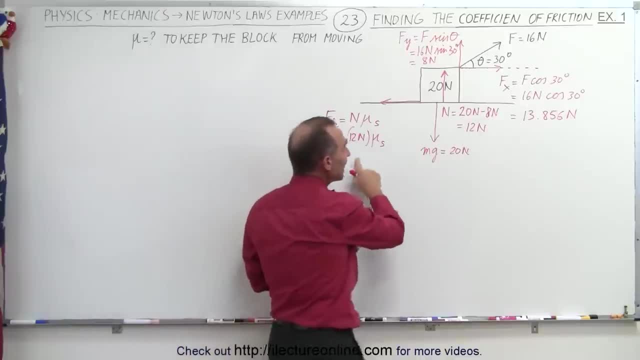 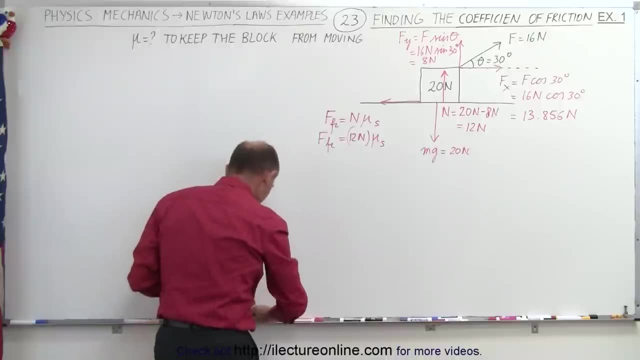 essentially, this is the maximum friction. force must be at least equal to the force in the x direction which we have right here. So what we're looking for is- and let me grab my black pen now- So what we want is to want the force, friction, to be greater than. 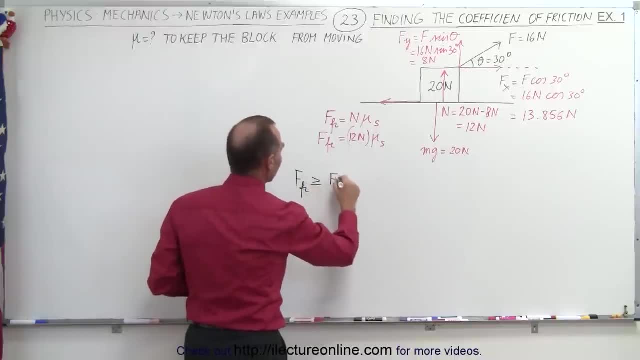 or equal to the force in the x direction that's applied And our friction force. we now know that's equal to 12 newtons times the coefficient of static friction And that must be greater than or equal to f sub x, which is 13.8..